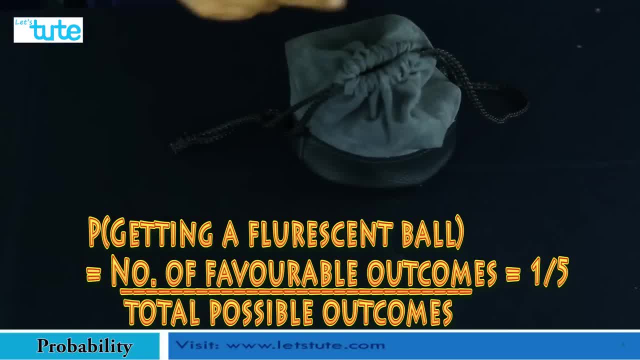 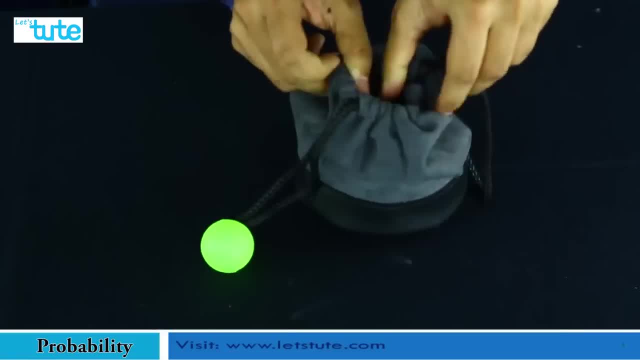 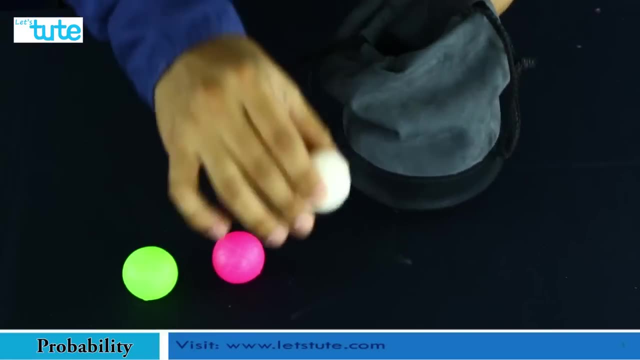 there is only 1 ball, 1 fluorescent ball, among these 5 balls, So the sum of the probabilities rule should satisfy this experiment. So now I said this has 1 by 5 probability. this will have 1 by 5 probability. this will have 1 by 5 probability. this will have 1. 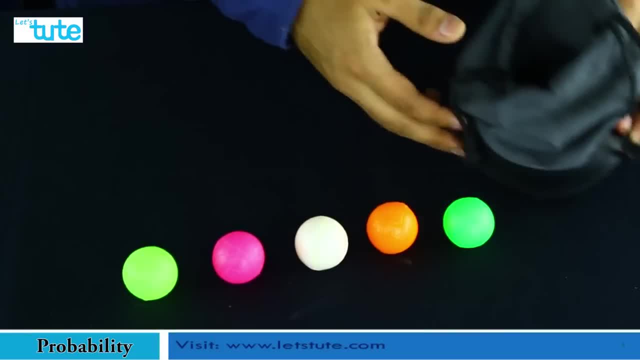 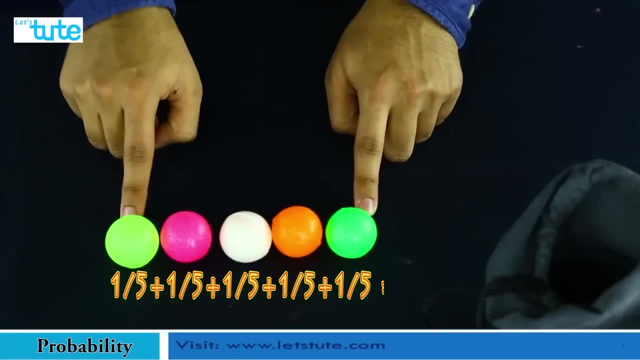 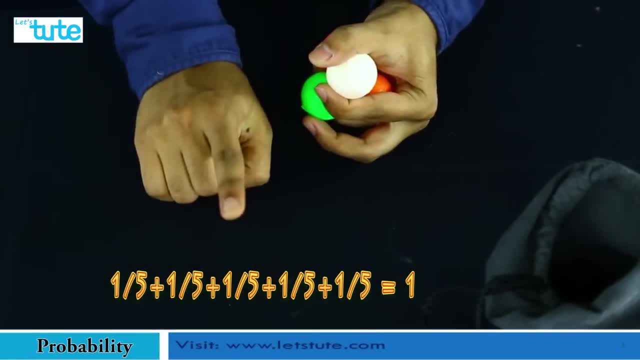 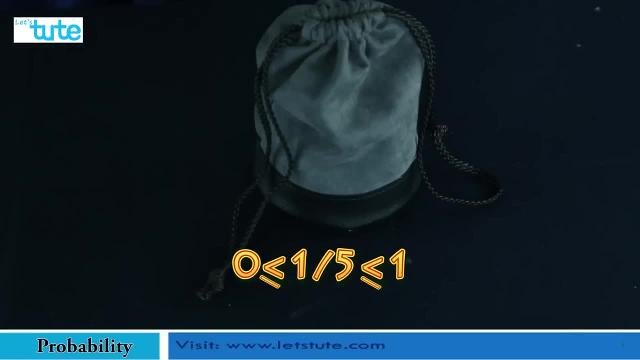 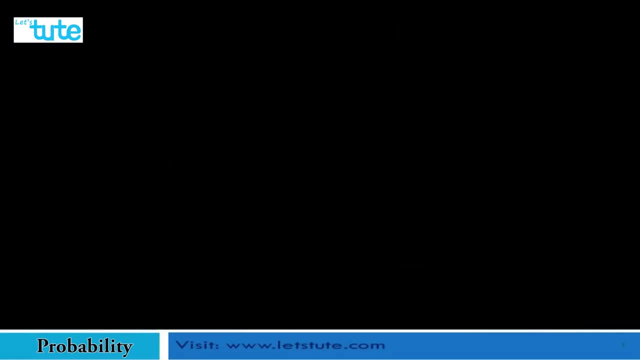 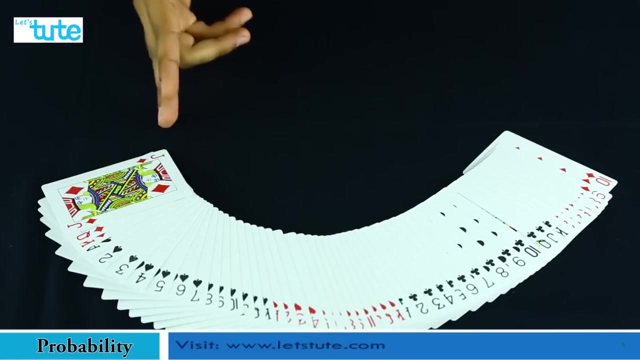 we are going to get probability equal to 1.. So this satisfies the sum of probabilities rule, and also 1 by 5 falls between 0 and 1. So it again satisfies all the rules. So the ball experiment is over. In a pack of card we have 52 cards in a deck and that forms: 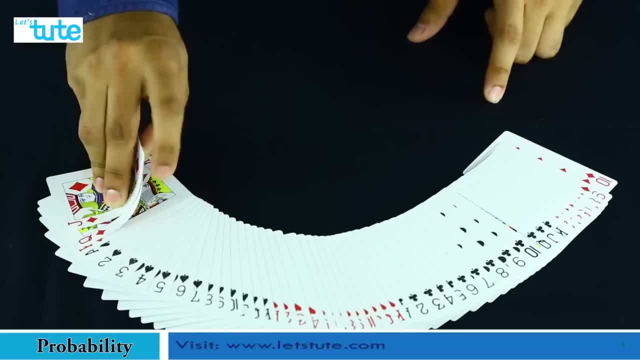 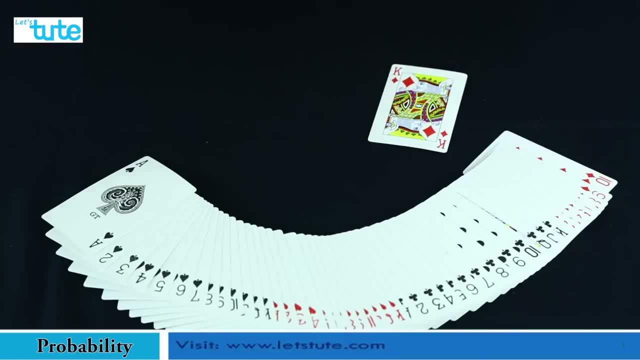 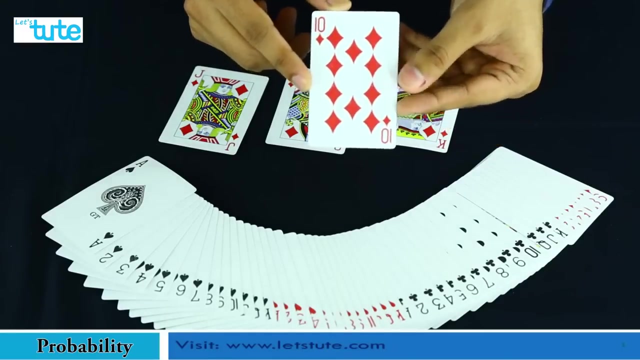 one pack or one deck In that we have three face cards, namely a king, a queen and a jack. These are the three face cards that we have, And we have four suits and each suit is represented by a shape or a color. We have one suit called diamond and this is red in color. We have 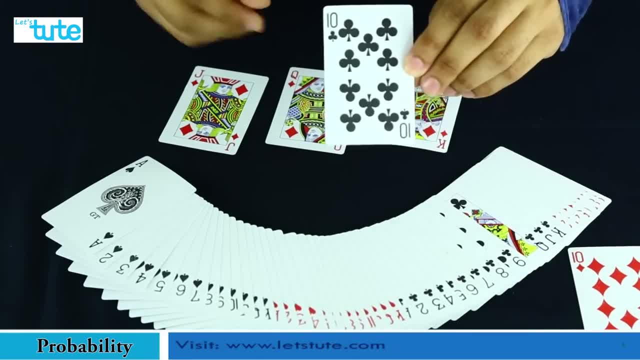 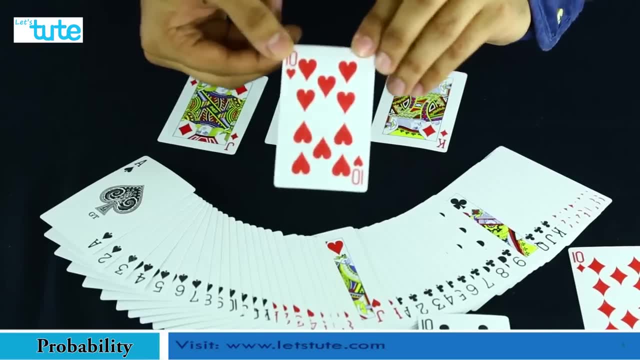 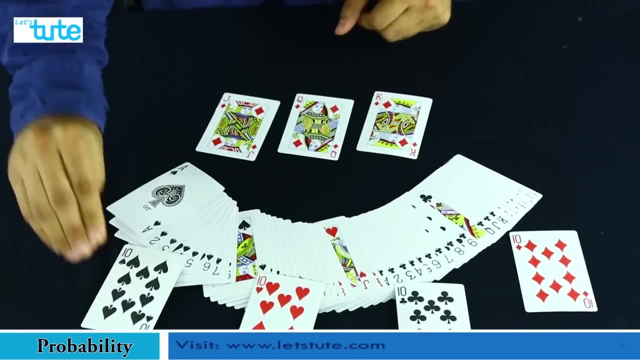 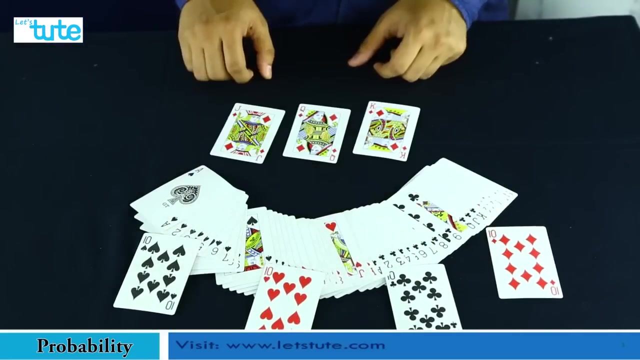 one suit, gloves, which is black in color. We have one suit called heart, which is again red in color, And we have one suit, spades, that is black in color. So the spades and the club is black in color and the heart and the diamond is red in color. There are four suits with three. 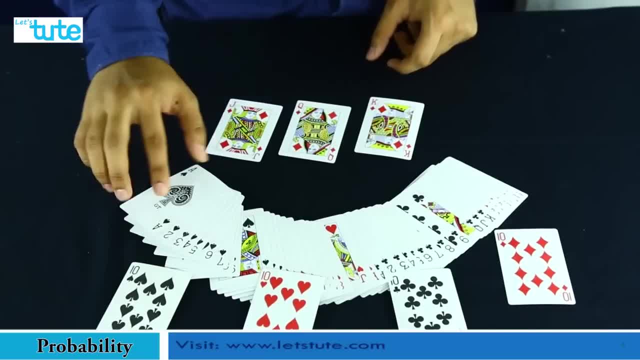 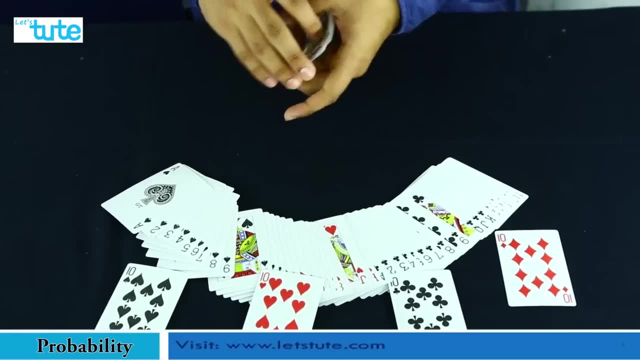 face cards and the other numbers are ace, 2,, 3,, 4,, 5,, 6,, 7,, 8,, 9 and 10. all right, So this is how the number goes. Now suppose we have this color and the number goes like: 8,, 9,, 10,, 11,, 12,, 13,, 14,, 15,, 16,, 16,, 17,, 18,, 19,, 20,, 21,, 22,, 23,, 24,, 25,, 26,, 28,, 29,, 30,, 31,. 29,, 31,, 32,, 33,, 34,, 34,, 35,, 36,, 37,, 38,, 38,, 38,, 39,, 41,, 42,, 43,, 49,, 41,, 42,, 43,, 41,, 42,, 42,, 44,.